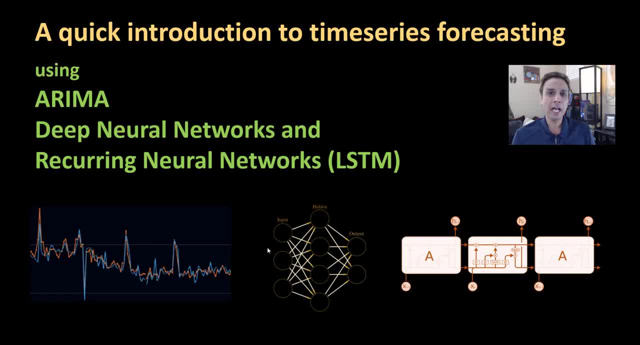 Hi everyone, welcome to my YouTube channel, and until now, we looked at primarily a lot of image analysis and data analysis when it comes to Python, and we looked at regular type of data, but part of the data that you will be working with, or I should say the type of data that you will. 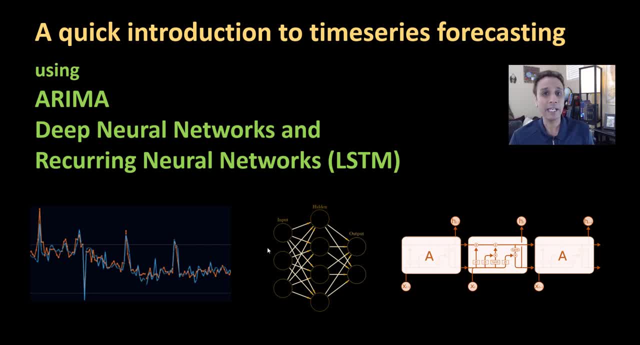 also be working with is a time series type of data where, obviously, as the name suggests, time series is where your signal or information is a function of time. So, whether you're in research or finance or any other fields, you may- or I should say you will- run into time series and you may be. 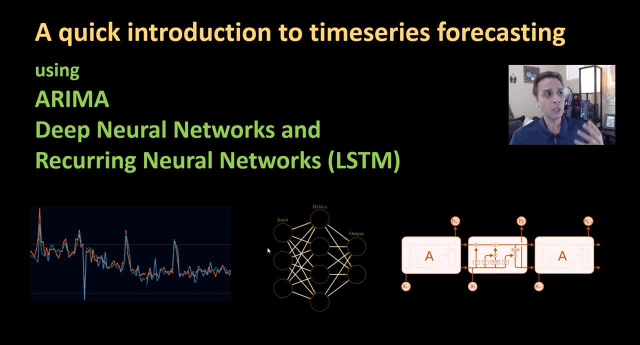 tasked with forecasting based on this time series data. So in this tutorial I'm going to provide a quick background of time series. In the next tutorial, let's actually load a data set and explore using Python. and in the three following tutorials or videos I'm going to use: 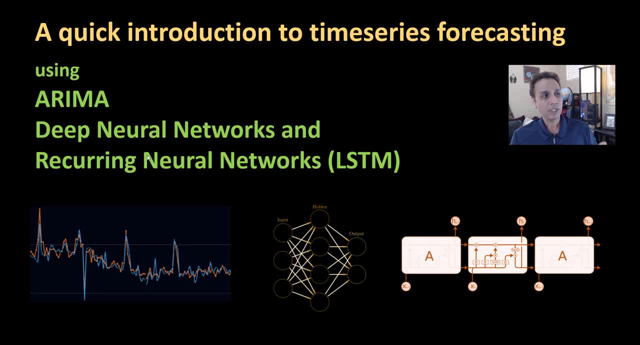 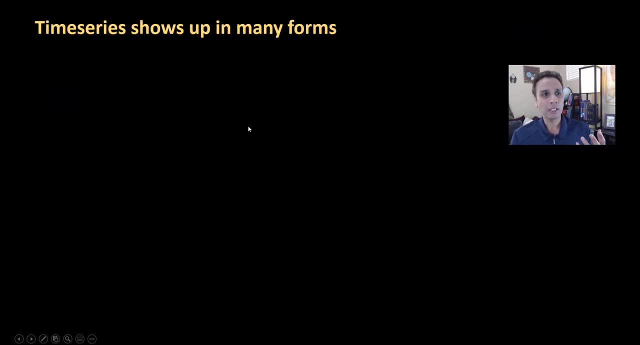 or cover ARIMA, deep neural networks and recurring neural networks, of course, using Python, and use these three approaches for forecasting purposes in, you know, using a time series. So let's first of all look at where you will, you know, run into this type of time series and, like I just mentioned, 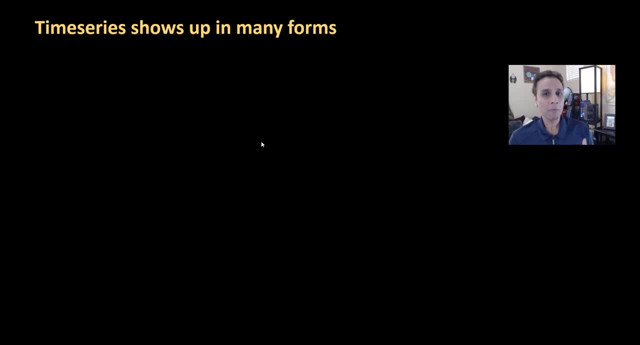 it doesn't matter what field you are. you probably will see time series at some point because things evolve based on time, as a function of time. So let's first of all look at where you will run into time. For example, if you are looking at cells and how cells are migrating or moving, I should say as: 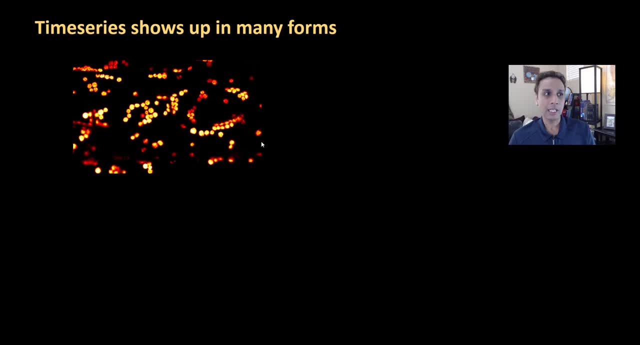 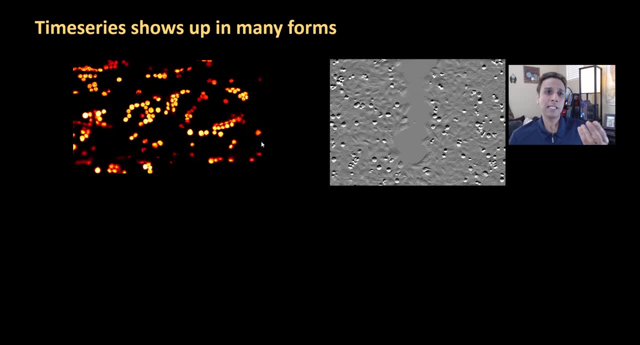 a function of time again. this is. this, technically, is time series. You are trying to get some properties out of this and then trying to fit those properties as a function of time. Same thing here. if you are seeing or imaging, this is our classic, you know, wound healing assay. If you are, 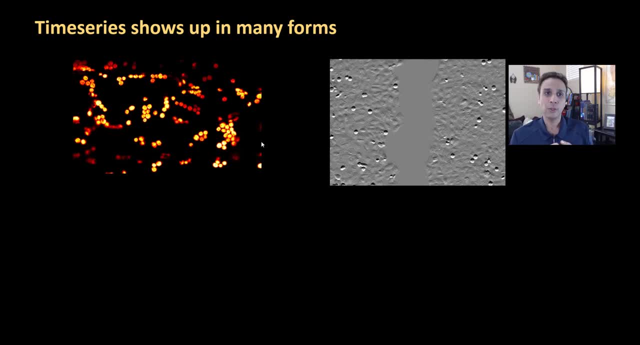 in life sciences. you know what I'm talking about. On the left and right hand side, you have cells and you can see that there are cells that are migrating or growing in that specific direction. So this is again a time series and in this case you can plot the scratched area, meaning as a function of time. 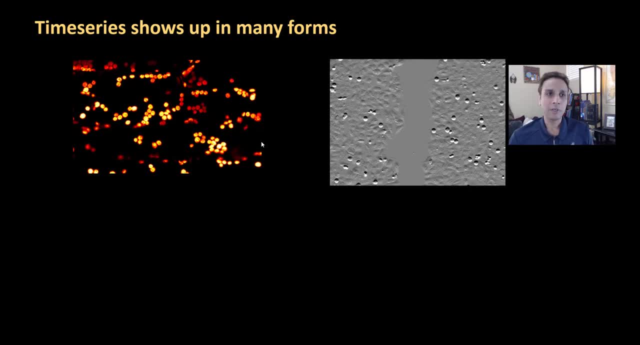 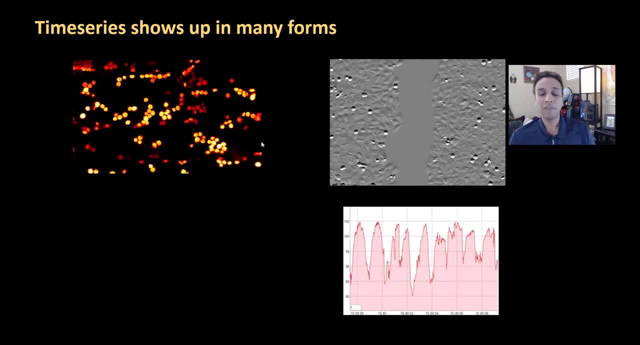 the scratched area goes down right. So this is again another example of time series. One more example of time series is you'll find that, as part of again this type of graph, you can interpret that in many ways. you know, I mean you can interpret that in many ways. So let's first of all look at 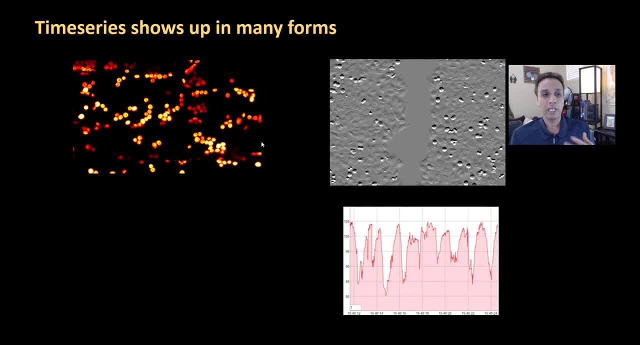 this graph. So let's first of all look at this graph. So let's first of all look at this graph, So apply this, or you get this type of response many ways, like one. you can think of stock market: okay, how is it going up and down, and hopefully it doesn't change by this much, but any signal that 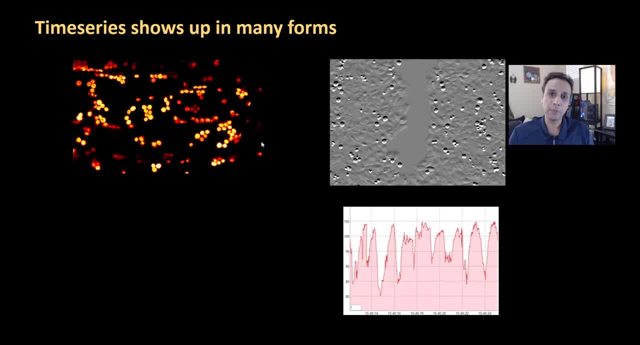 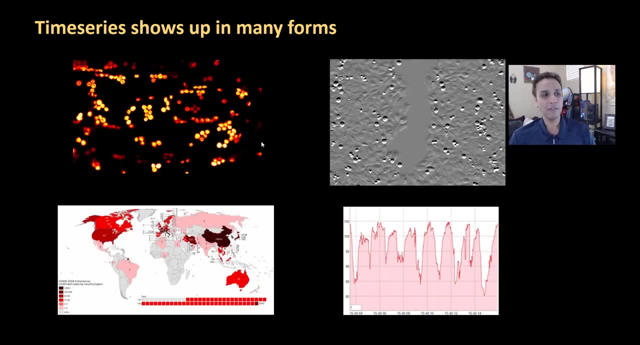 you're collecting, you know that can actually depend or fluctuate based on the time, and that's what I'm representing here and nowadays, of course, we are in the middle of COVID, so even if you want to look at the number of cases as a function of time, you know okay, in the beginning last December. 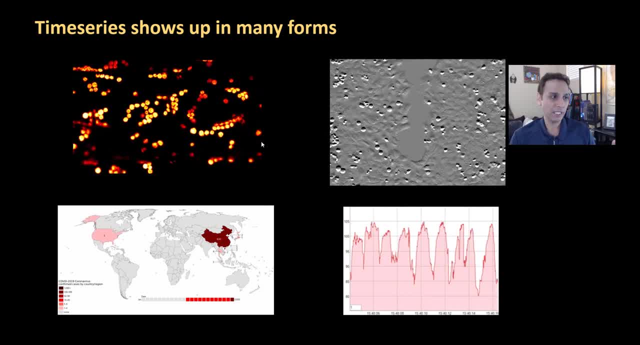 and then January, February, March, April, it started to spread to other countries, and so on. Now, if you want to quantify things, this is again time series. Now, why is time series different? Well, time series is different from other data that we have used in the past because in the past we 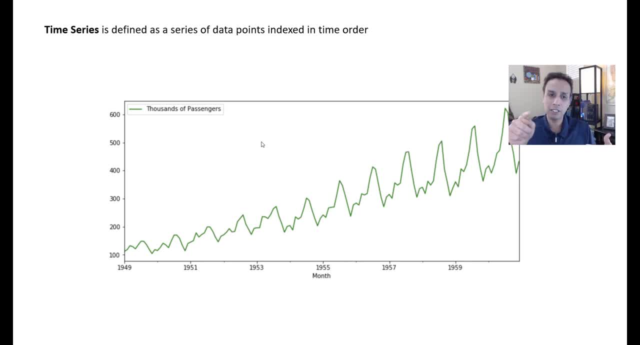 looked at a whole bunch of attributes and tried to predict: okay, is this a cat, is this a dog? or we looked at a whole bunch of data and said, okay, can we sell this or can we not sell this? yeah, But when it comes to time series, 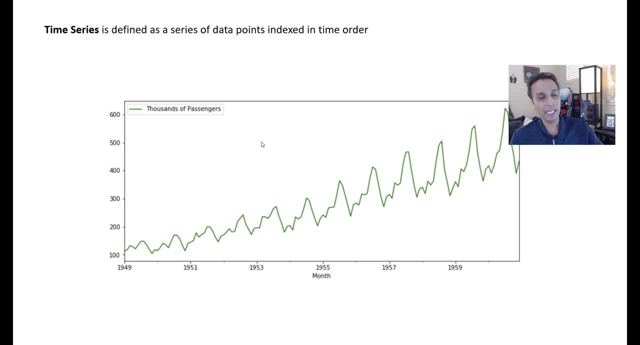 here. it's just a function of time. I mean again, I don't have to go through the definition, it's on the screen. you can see that the data points are indexed against time and the time can be year, month, millisecond. if you're looking at the number of alpha particles emitted per millisecond from a. 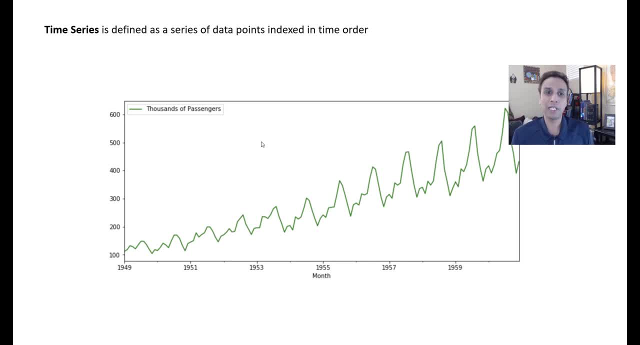 radioactive material, then of course now on your x-axis you have milliseconds on y-axis. you know the radiation. I guess it would be pretty random, so you would see a pretty you know random fluctuations per second. So if you look at the data points you can see that the data points are indexed against. 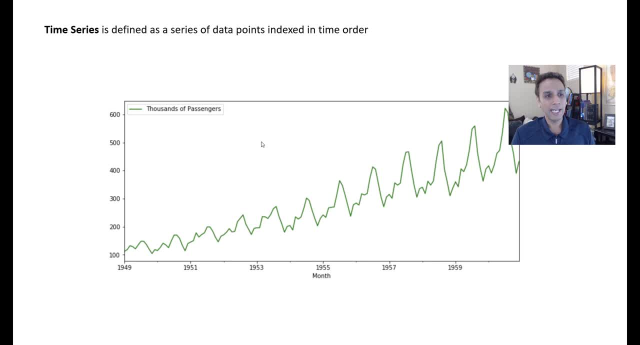 the time, and the time can be year, month, millisecond, if you're looking at the number of alpha particles for your actual signal. but if you're looking at airline passengers, which is what this data set represents, then okay, as a function of time, like per year or per month, how many passengers are? 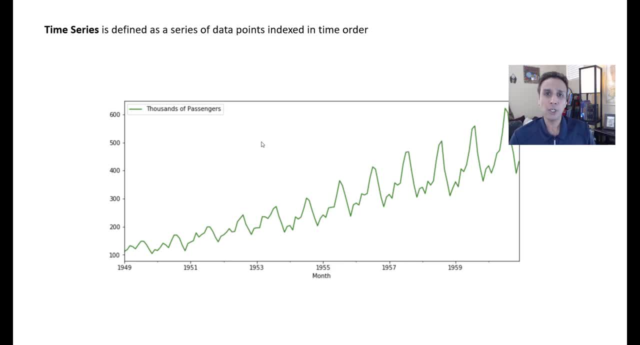 traveling. So this is basically the time series, and I know I'm pretty sure you know what I'm talking about here. now again, why are we talking about this in a separate context? because if you model this, then x-axis doesn't mean anything, it's just the time is increasing, right? the data is not correlated, typically, you know, with anything. 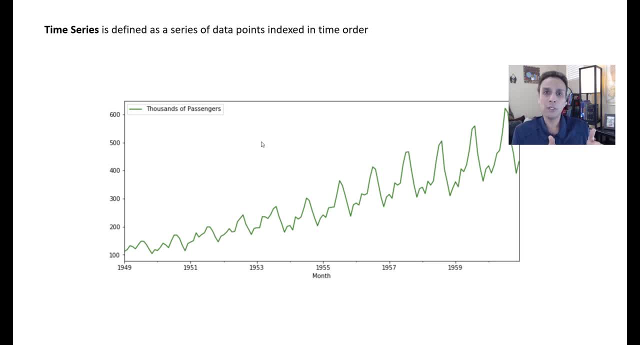 but itself, meaning if you look back one month ago and a month ago and a month ago, you'll see a pattern, but if you kind of correlate that with something else, you won't see a pattern. that's why our time series is different from other type of data that we have analyzed in the past, including 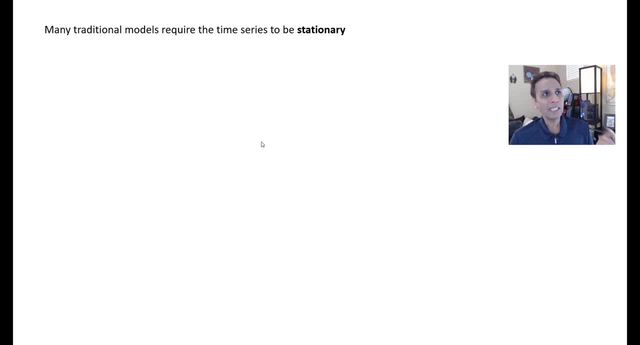 image analysis. Okay, so one thing I would like to mention. I don't want to go into too much detail about time series analysis. I hope you already have background, or, if not, maybe whatever little thing I cover is a good start for you. So most traditional models require time to be stationary. 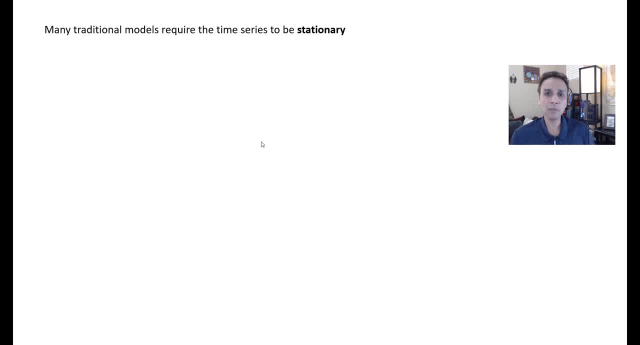 if you have used traditional models like auto regression, you know ARIMA or some of these traditional techniques, even Fourier transform based techniques. it requires the data to be stationary, otherwise how can you forecast if the mean and variance are changing? by the way, I should have defined what stationary is. Stationary-based data is the data that is used to predict the time. 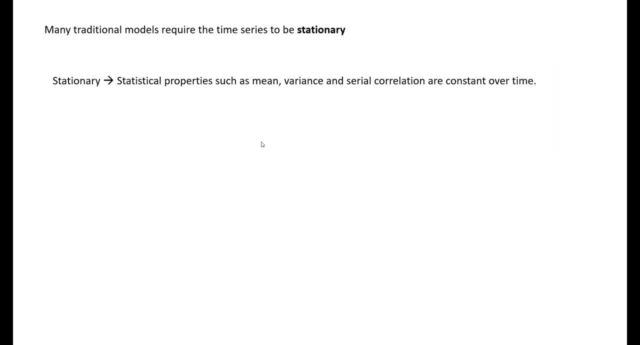 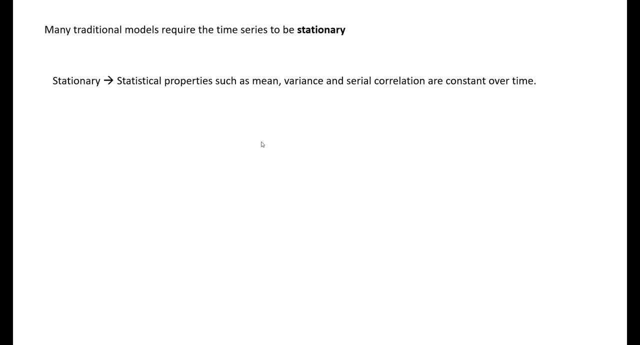 you cannot predict it. okay with traditional models, but the newer approaches, whether it is LSTM's or approaches like SaRIMA, for example, they are designed to work with some of these data sets that are non-stationary. now, what do I mean by stationary? you can see a quick graphical representation on the screen. on the left hand side you have 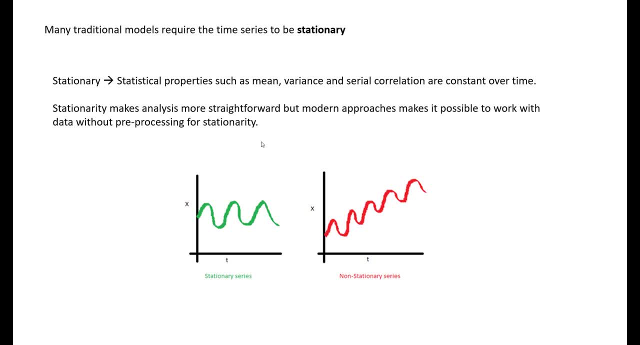 a stationary series where you can see: yes, of course it is fluctuating, but you can see that it's. it's doing that in a predictable way. non-stationary- this is just one example, but non-stationary also means things are changing in a different way as as time goes on, and so on. 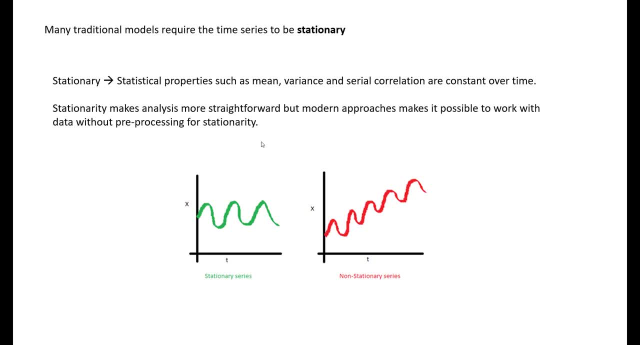 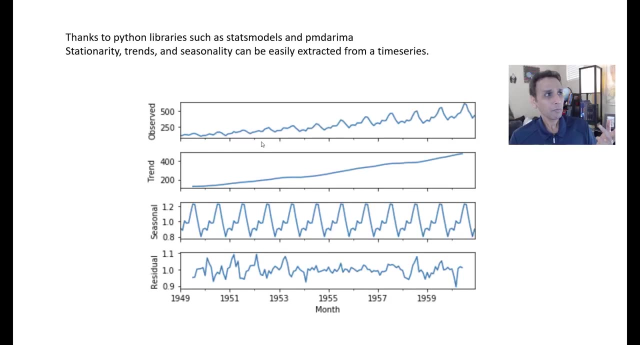 you can correct for these and then use the traditional methods, but you don't have to correct for these if you pick the right approach. that's the reason i wanted to cover arima, or sarima, and the deep neural networks and lstm for this, uh, for this, demonstration purposes now, uh, like i said, 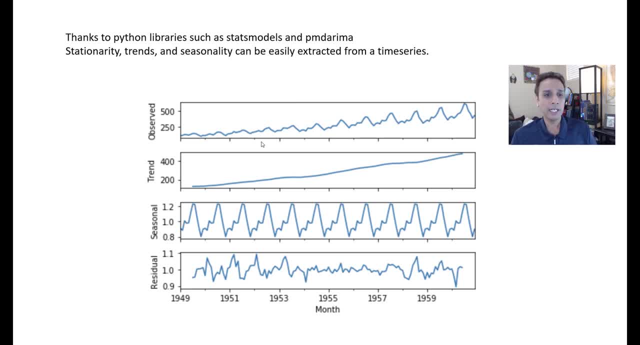 thanks to these, some of these python libraries. i mean this used to be, uh, something that you need to code or do it in excel you know a lot with with a lot of effort, but now with a single line, uh, in stats models, for example, is a python library that i absolutely love for this type. 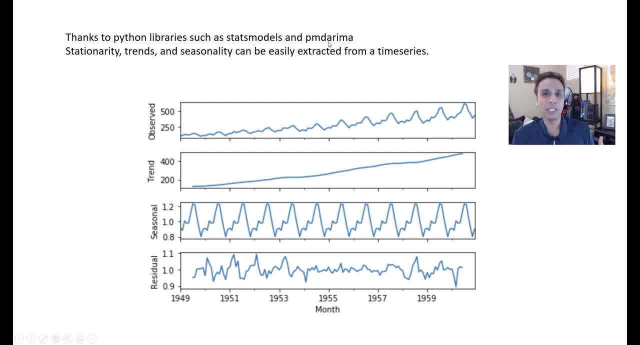 of application. so i'm going to go ahead and show you how to do that, and i'm going to show you how to work. also, pmd arima is another one that actually works very well. so with a single line of code, you can actually take your actual observations and obtain a trend. trend is as: 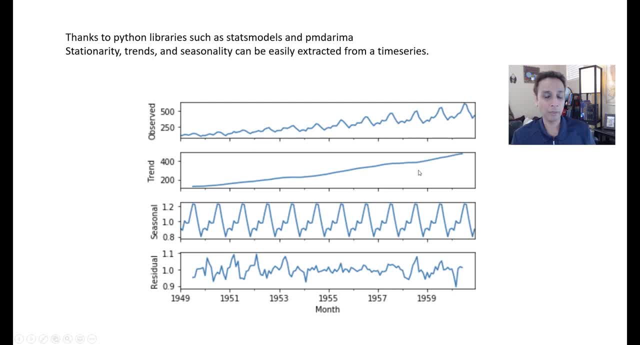 the name suggests it's a trend. how does the data trend as a long period of time? so, as you can see, the trend is more people are flying. as you go from 1949 to 1959, the number of people that are flying, uh, they're going up. but then, on top of that, you have seasonality, which means okay, in summer, more. 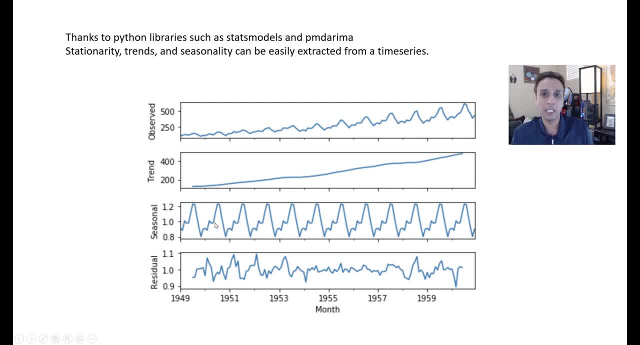 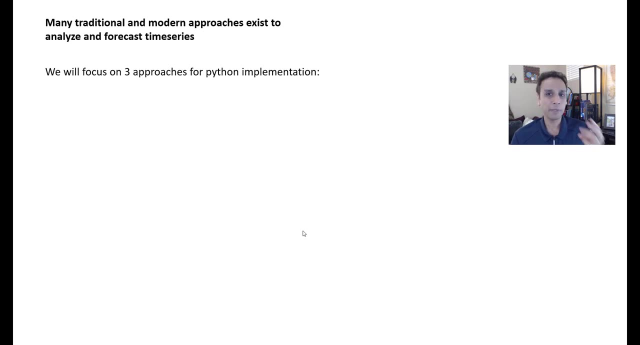 people travel. in winter less people travel, or i just made that up, but that could be the trend here. okay, during holidays people travel, or during summer vacation time, people travel. so, uh, now, uh you, there are many traditional and modern approaches, like i already mentioned, but i'm going. 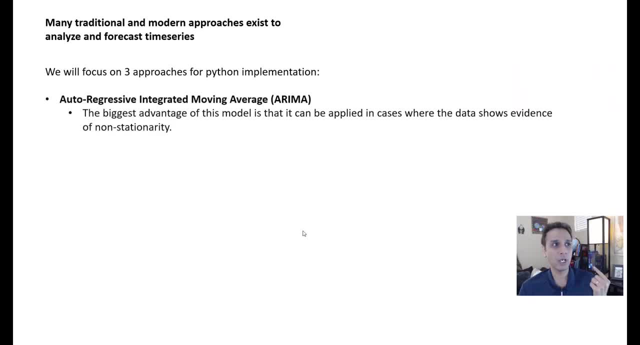 to focus only on the three primary approaches. one is auto regressive. it's called arima. ar stands for auto regressive and ma stands for moving average. these two are two techniques. now we are going to put them together and put integrated in the middle. and again, it's very widely used. that's why. 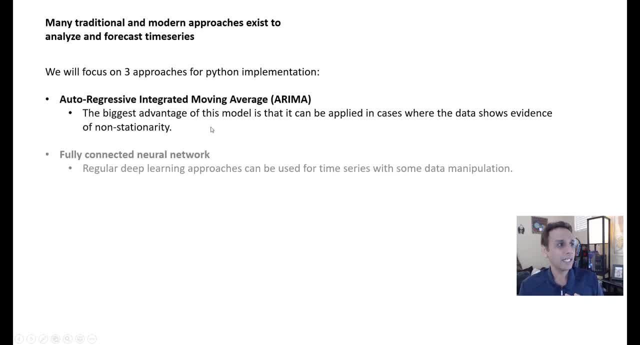 I'm not talking about anything else other than this, and the other one i'm going to talk about is fully connected neural networks. this also works fine on most types of data sets. because we have used neural networks in our past videos, i thought of actually just go ahead and use it and see how. 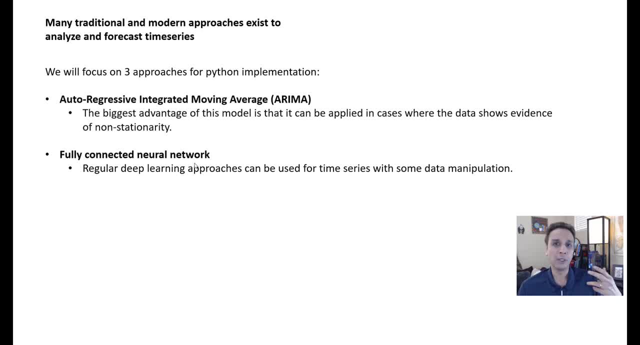 time series data can be fitted to a model and then that model can be used for forecasting. Exactly same approach for LSTM. LSTM is again another neural network-based approach, but it's in fact a part of something called recurrent neural networks. Again, I'll take some time, at least create a video talking about. 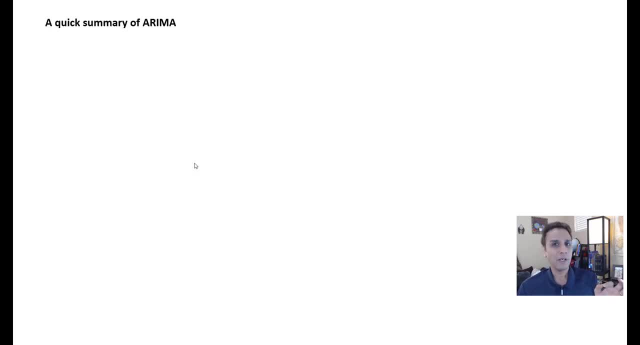 LSTM. Okay, and ARIMA itself. maybe, if you're coming from scientific background, you're probably not used to what this is. Again, if you have taken any courses in business or even in statistics, you may have you know. looked at this ARIMA. like I mentioned, it's AR plus MA, integrated with 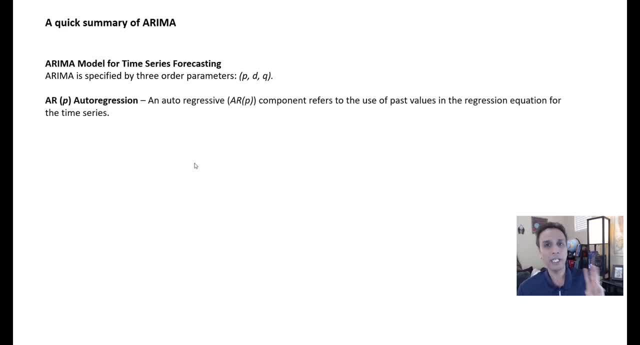 an I term right there. There are three parameters: PD and Q. Again, I don't want you to get confused here, but I want to introduce this PD and Q because later on, when we talk about it, when I'm doing okay, my P equals to one and D equals to one and Q equals to two or something you would. 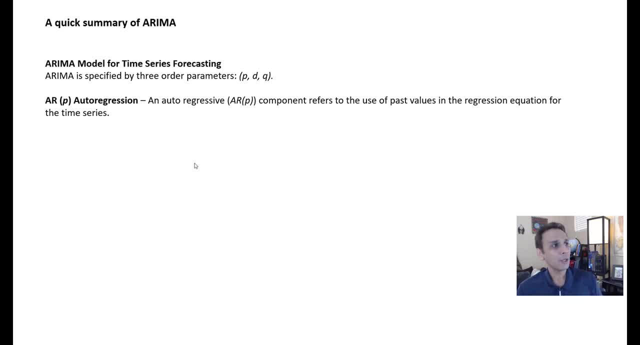 at least have an idea of what I'm trying to do there. Okay, so AR stands for autoregression, like I mentioned, and we have a term called lowercase p. You will also see uppercase P, depending upon the seasonality, but let's not get into that yet. The P component is the one that 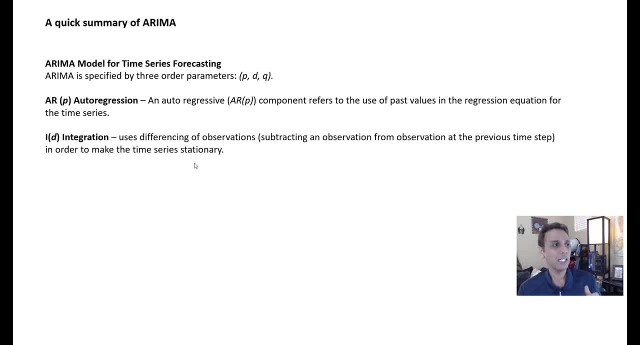 kind of controls the autoregression or defines the autoregression part, and I is the integration which is basically, it uses the differencing of observations, okay, and this is represented by. you'll see, moving average is represented by a parameter Q. Now there are again. I just used 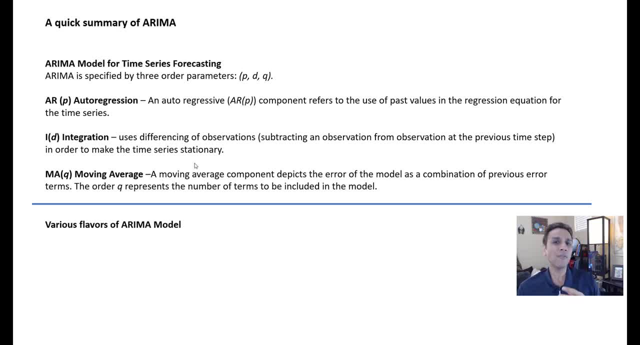 the term ARIMA, but this is a general approach, but there are a few flavors of ARIMA. like you, this is basically non-seasonal, autoregressive integrated moving averages. if I just say ARIMA, which means if you have any stationality, seasonality, you know, you kind of take care of it. 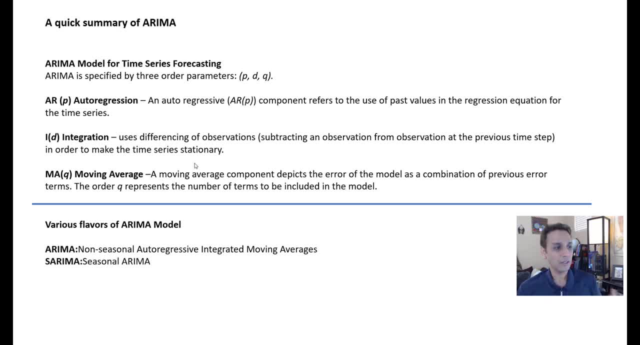 during your pre-processing of data. Now there is something called SARIMA S-A-R-I-M-A, so this is designed to deal with seasonal aspects. so most of the time I use this, and it's built on top of ARIMA, obviously, and SARIMAX is another one, and I'll also use the auto ARIMA in one of the 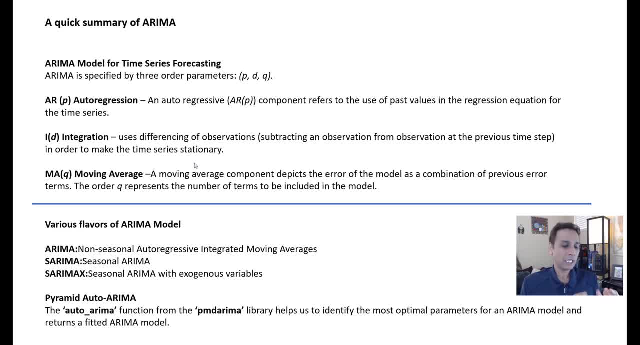 libraries, because it actually tells us what P, Q and D values are appropriate and what model is appropriate based on the data. So I'll introduce all of this, but then, when it comes to Python, it's literally very straightforward. 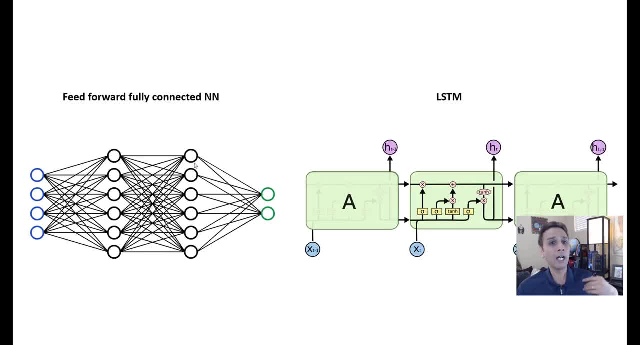 So please, please, watch that video. Okay, now we just covered ARIMA, Let me just quickly talk about feedforward fully connected neural networks. Again, we know what these are. These are, you know, these neural networks that are actually connected, so from every neuron to every other neuron. 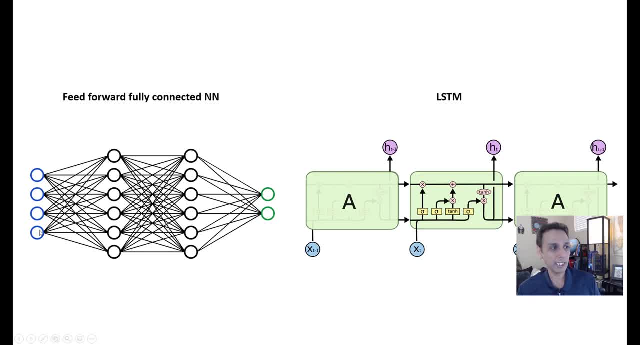 and finally, we have like two outputs. For example, if the input is all the features describing a cat and the output can be a cat and a dog, and cat with a probability of, let's say, 0.8, and dog with a probability of 0.2.. 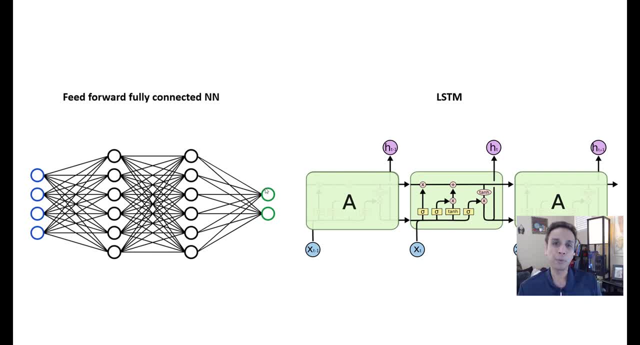 each point we say: okay, it is highly probable that the input image is a cat. Of course, now we try to use this classification or convert that classification engine into a forecasting engine for time series. LSTMs again, if you see a graphic like this, it refers to a LSTM and LSTM. 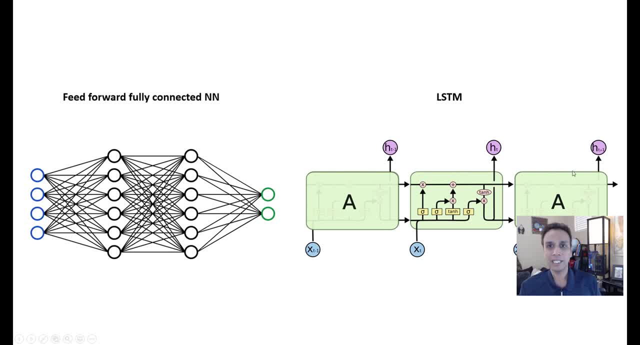 has you see this thing at time T minus one and that thing at T plus one. What that represents is: yes, I'm doing something here, but I'm taking the impulse from the input image and I'm taking the information from the previous- uh you know- step and i'm also handing information to the next step. 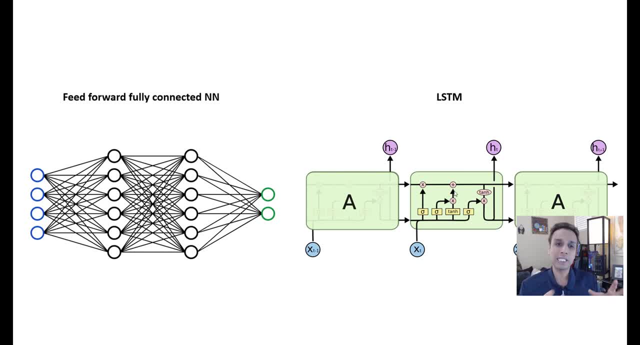 this basically means lsdm is designed to work with sequence type of data, which is time series, of course, but also natural language processing. when i say the term processing, i know that, okay, after p, i have r, after r, i have o and then c, and then it should naturally know what should follow.